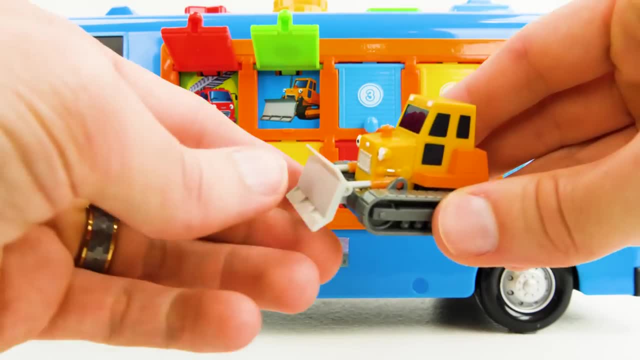 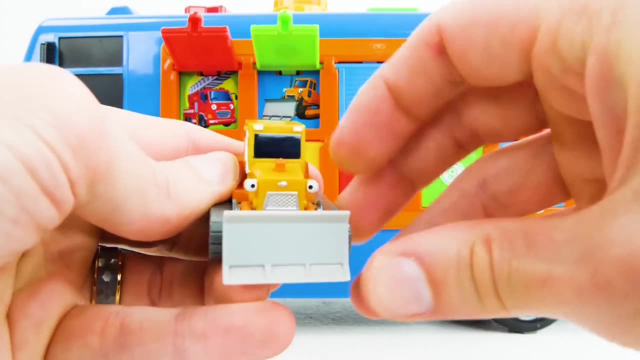 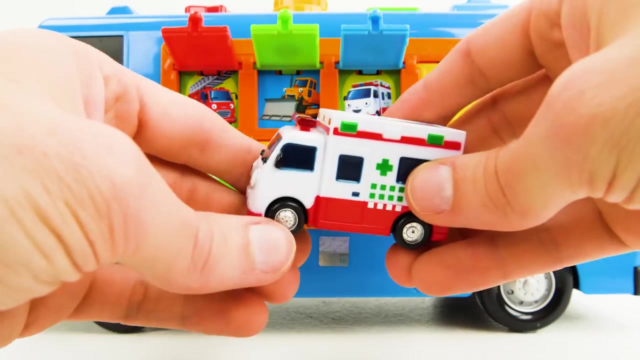 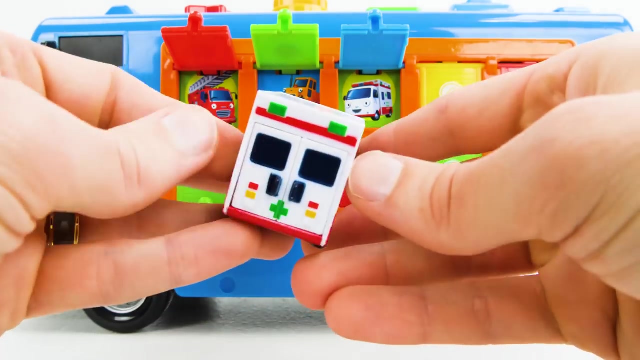 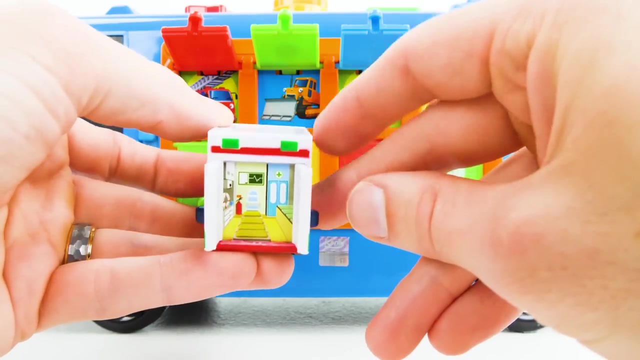 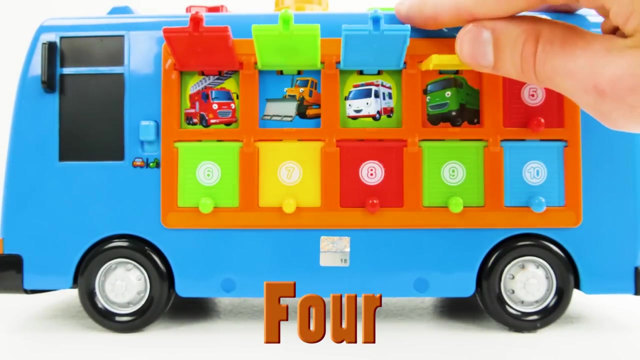 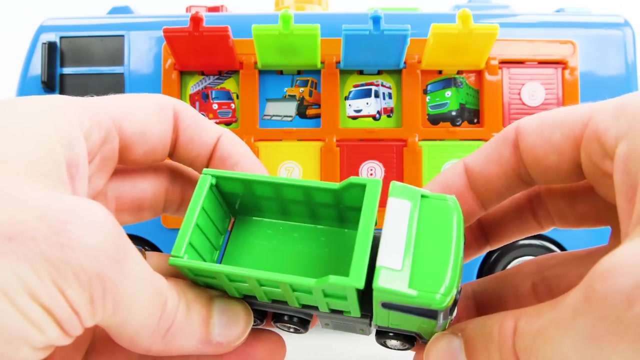 Two: Bulldozer: A bulldozer can use its shovel to push dirt. Three: Three: Ambulance: An ambulance takes people who are hurt to the hospital. They have a bed inside for people to lay on. Four: Dump truck- Dump truck- A dump truck is really good at carrying things that are heavy. 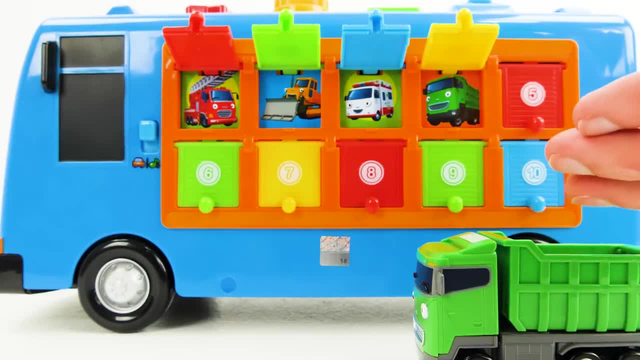 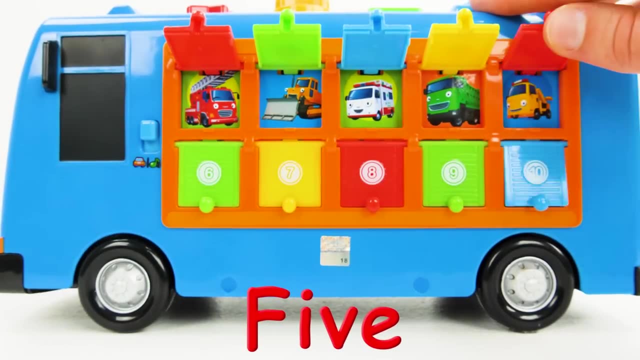 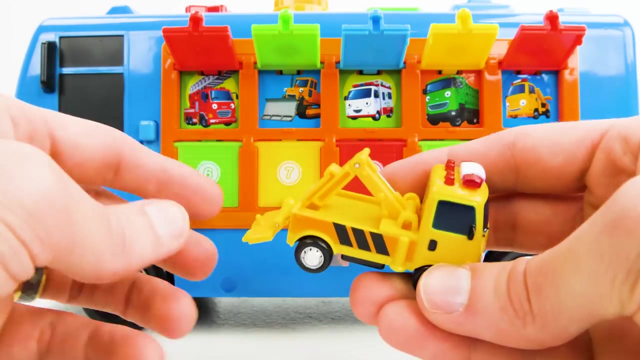 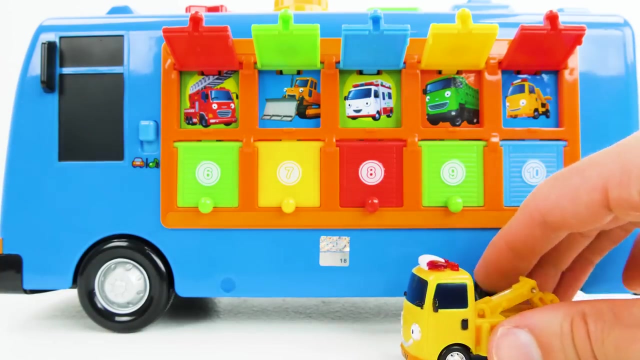 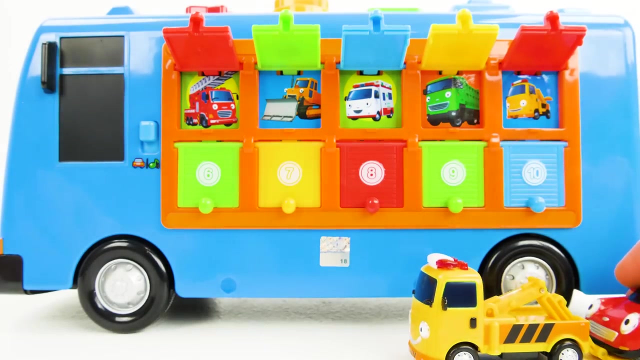 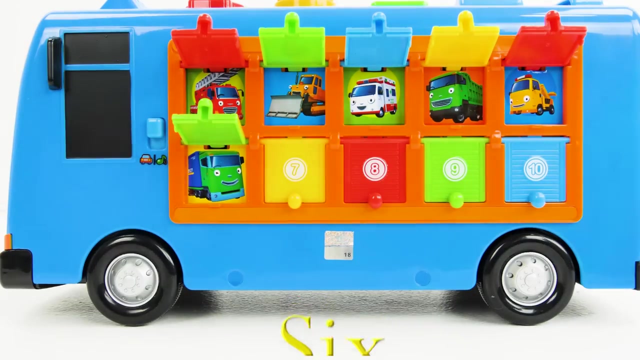 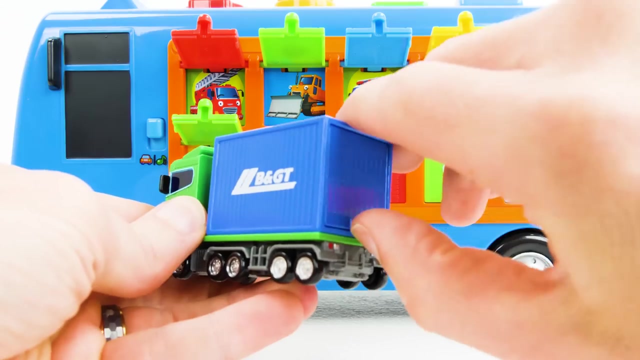 Let's load this one with gumballs. Five: Tow truck: A tow truck can pull a broken car to a mechanic. This red car is broken. It needs a tow truck. Six: Hauler: A hauler can transport things from one place to another. 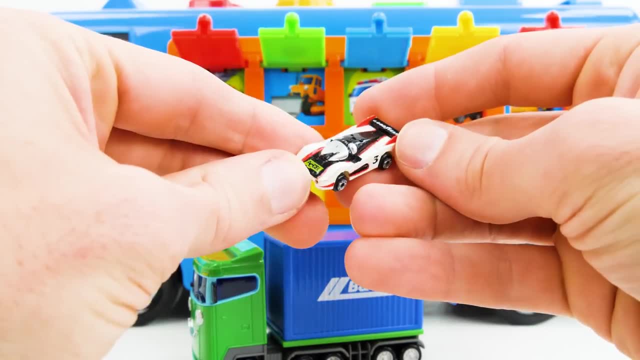 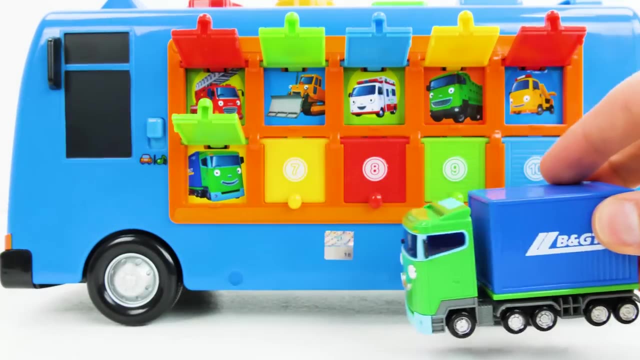 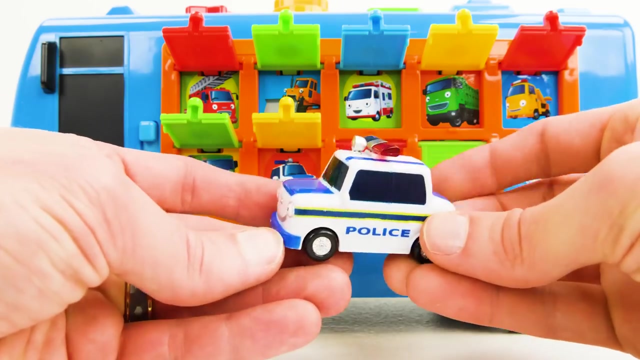 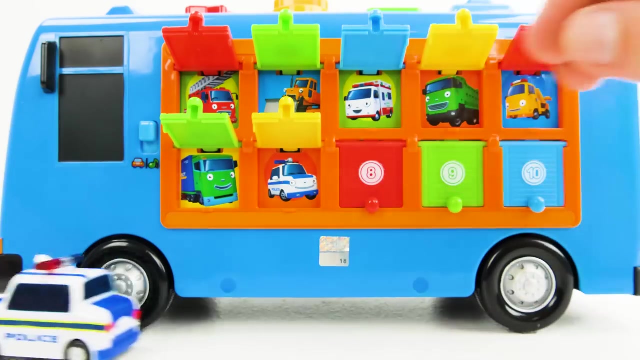 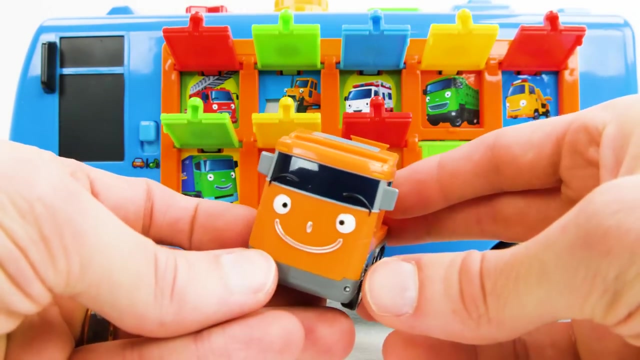 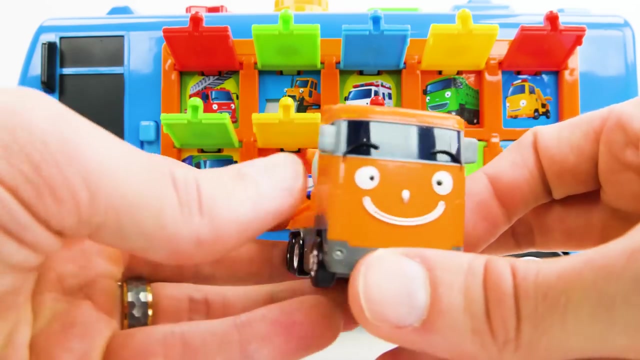 This one has a race car inside. Let's put the race car back inside the hauler. Seven: Police car. A police car makes sure everyone follows the rules. Eight: Cement mixer. A cement mixer mixes concrete for the sidewalk. How many cement mixers have you seen? 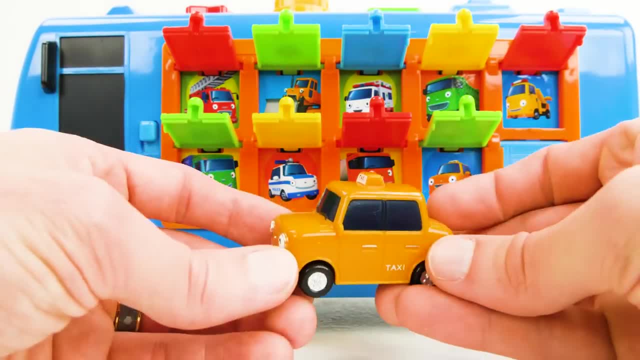 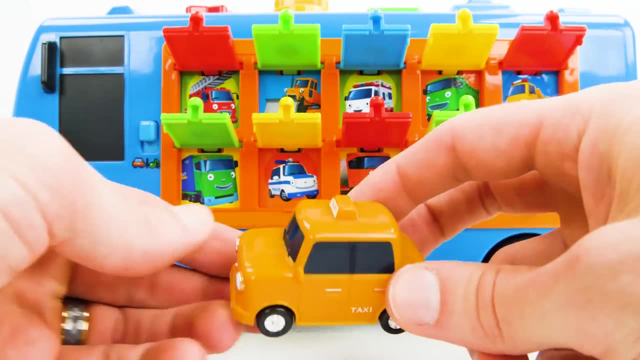 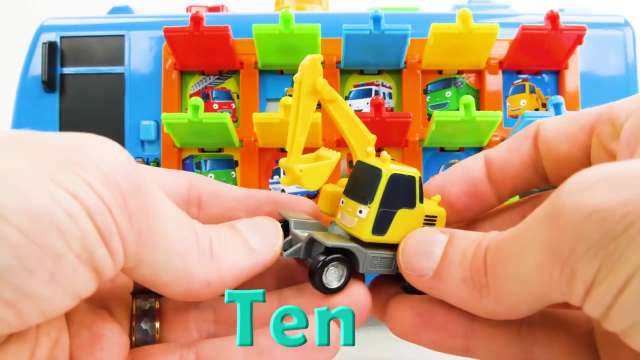 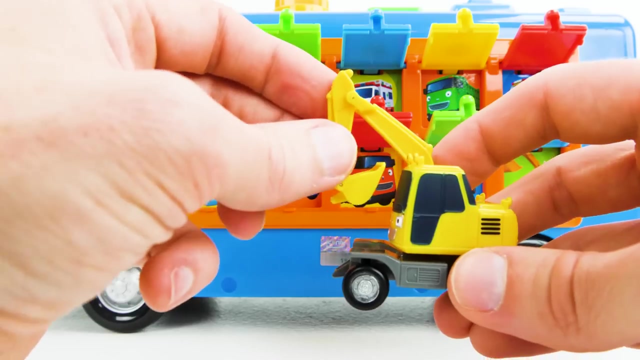 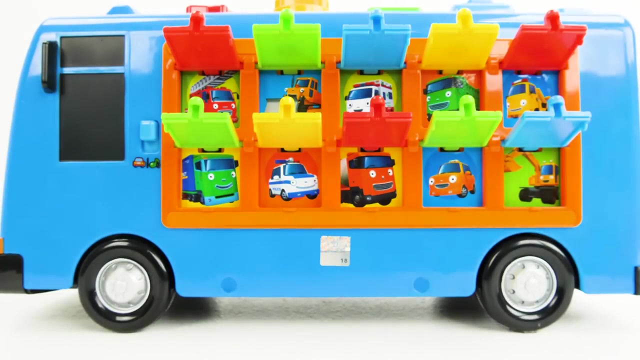 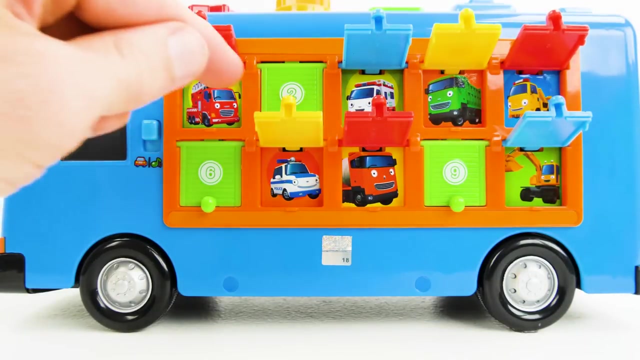 Nine Ten Taxi: A taxi helps people who need a car. Ten Excavator: An excavator uses its bucket to scoop dirt. It can turn and it has a scooping arm. Let's close the green windows, Now the yellow, Blue ones. 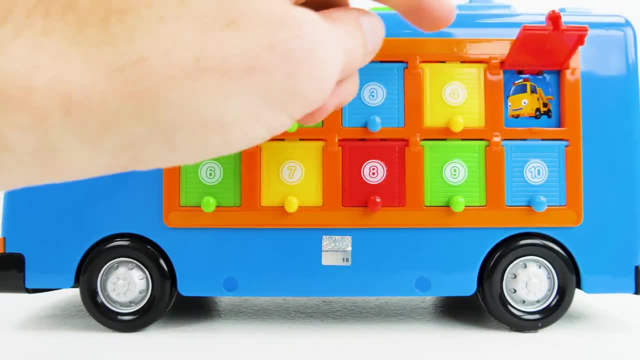 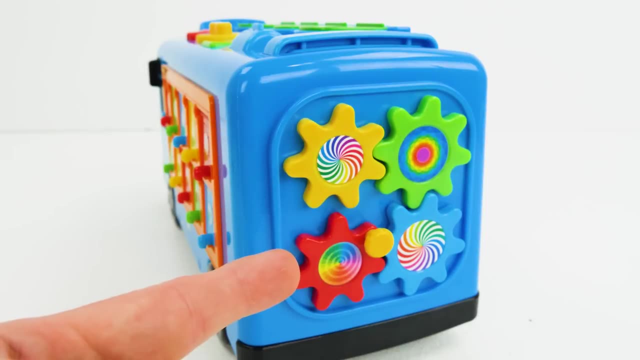 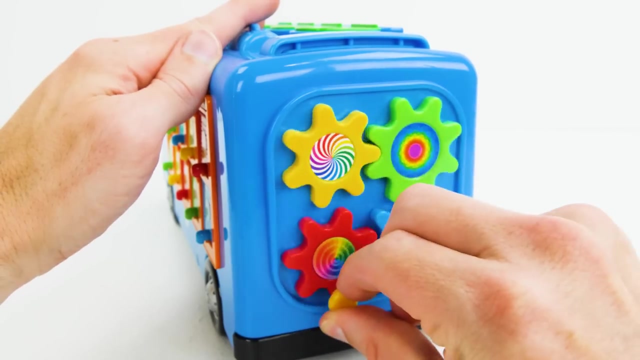 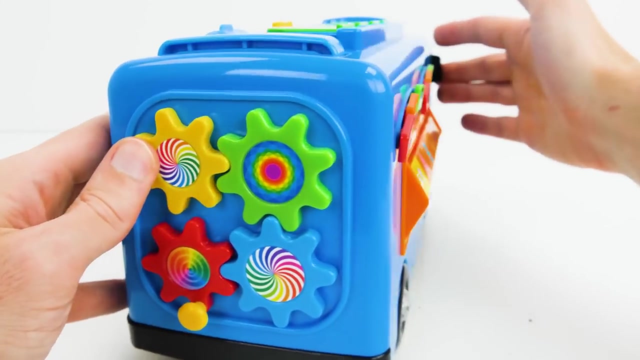 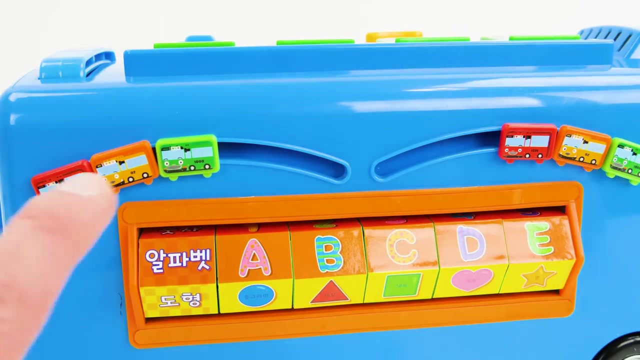 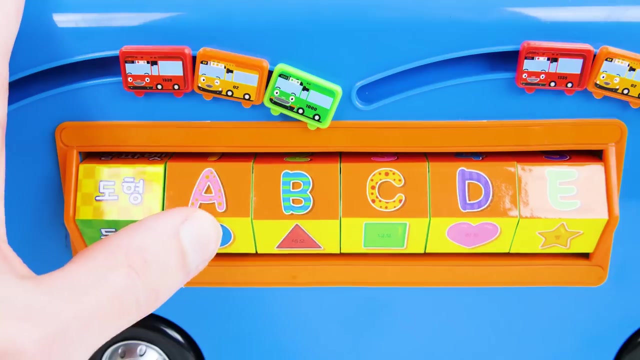 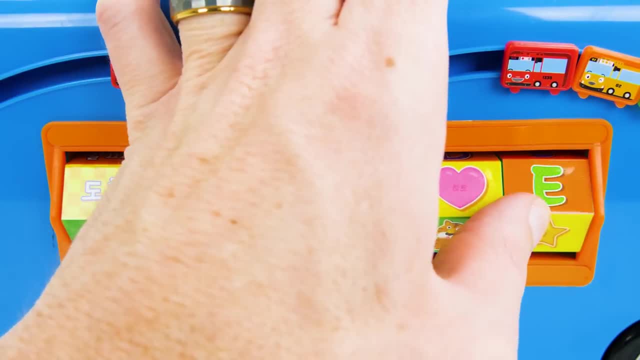 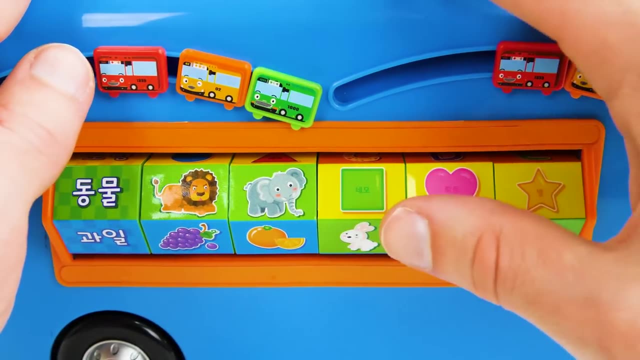 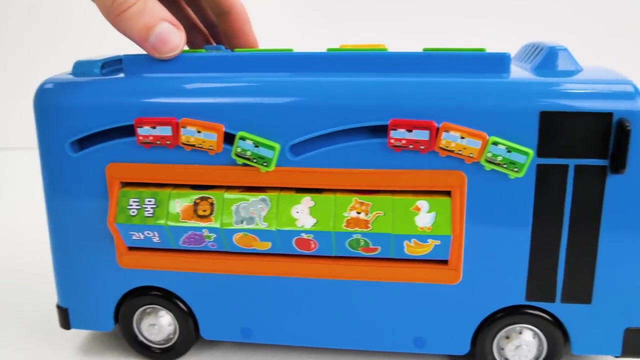 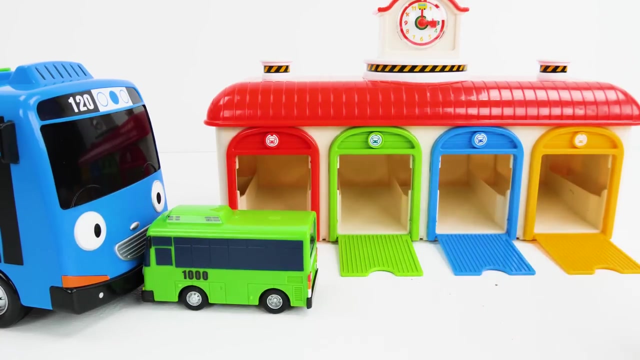 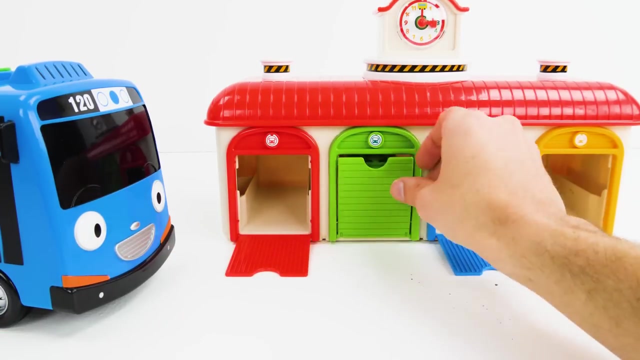 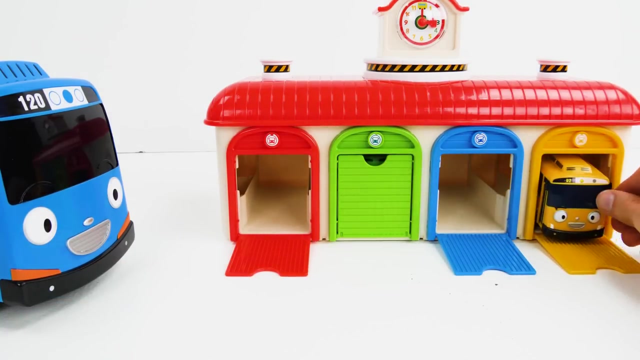 Square. Heart. Star Animals- Lion, Elephant, Rabbit, Tiger, Duck. Tayo's going to his garage. Let's match the buses. Green Bus: Look out, Tayo. The green bus can go in the green garage. Yellow Bus: Let's put the yellow bus into the yellow garage. 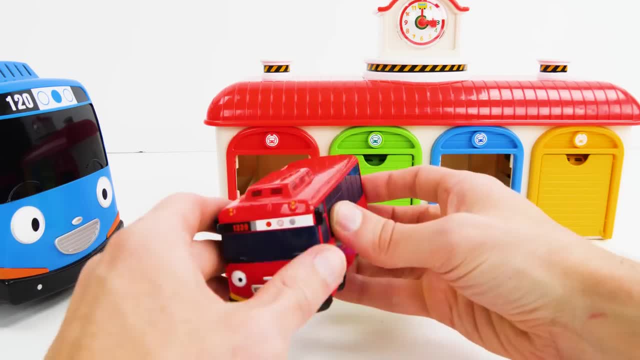 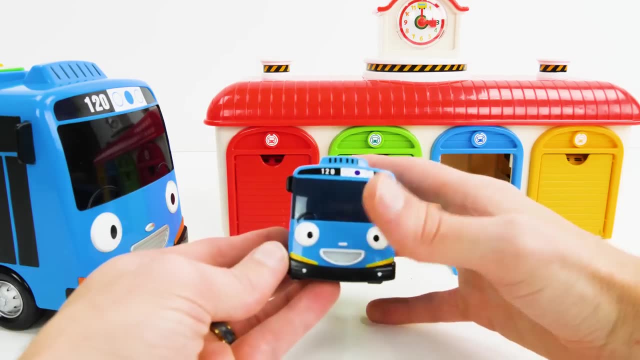 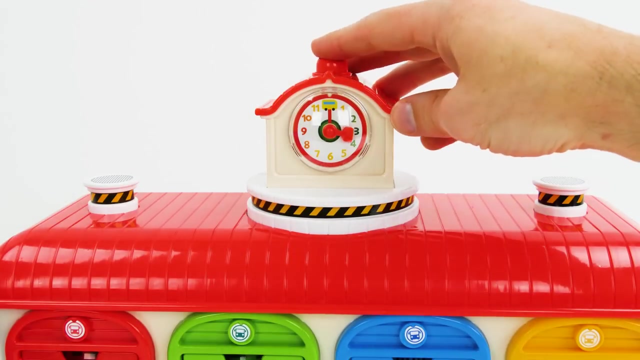 Red Bus. Where does the red bus go? Right here, You're right. Great job. The last bus is blue, just like Tayo. It goes in the blue garage. Let's set the time. Now we can check the garages. 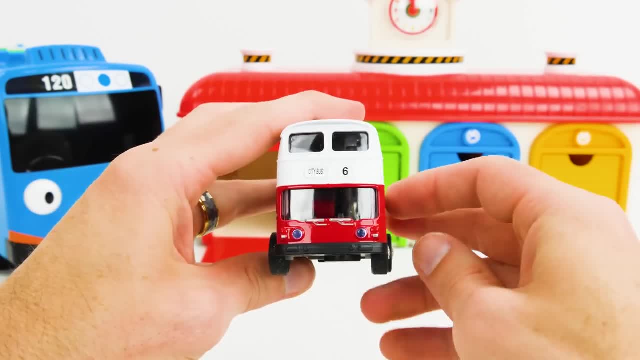 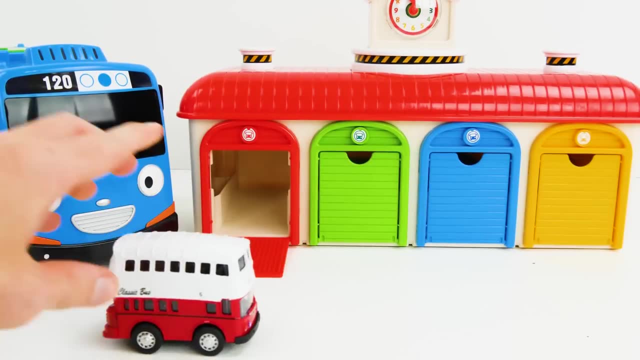 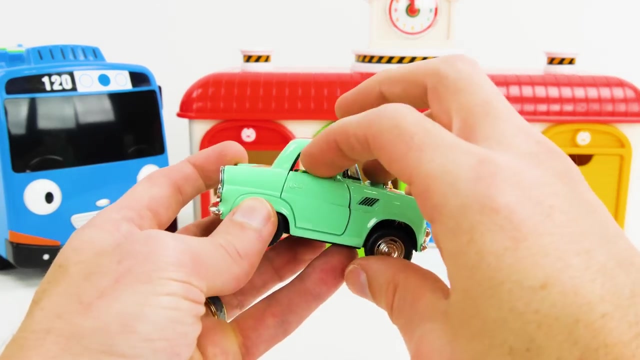 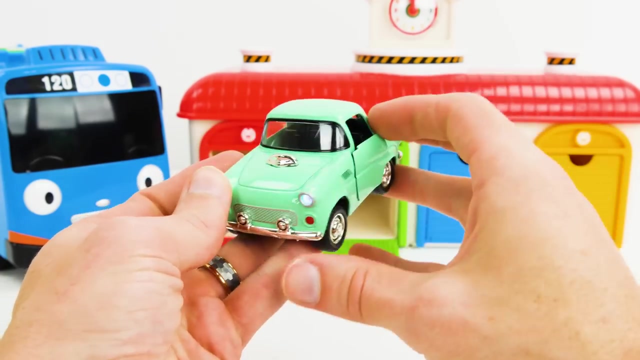 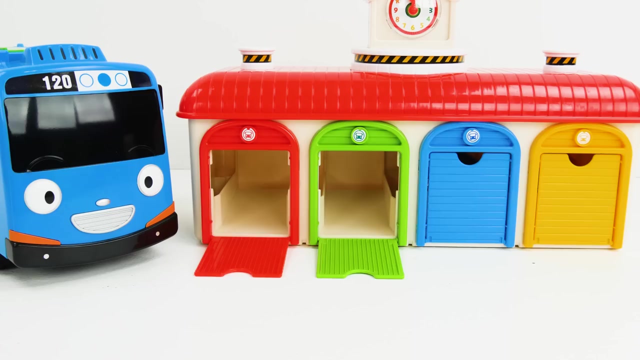 Oh look, It changed to a red and white double-decker bus. Now the green bus turned into a light green classic car. A classic car is really old. Let's see what our blue bus turned into: It's a blue sports car. 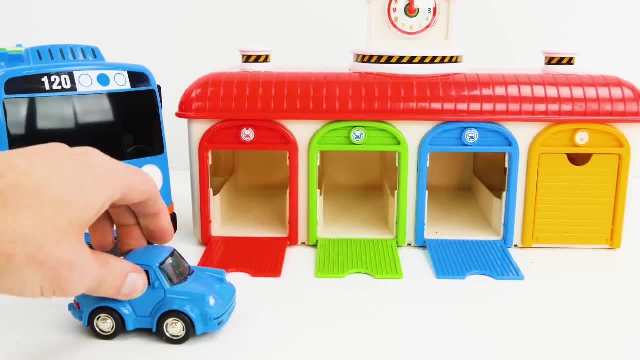 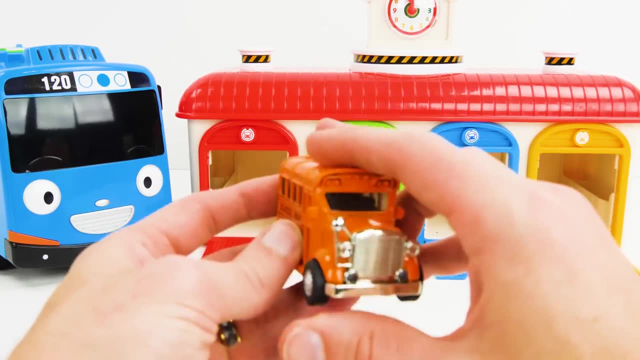 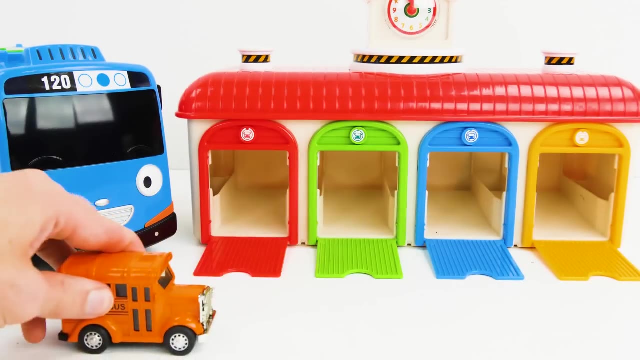 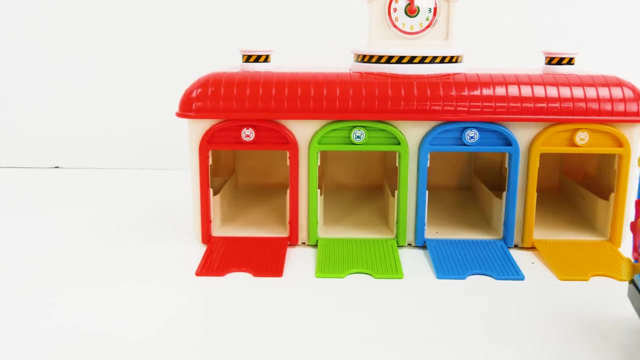 Sports cars can go fast. Our last bus turned into a school bus. Do you ride a school bus to school? Tayo had fun playing with you. Did you have fun too? Yes, I did.